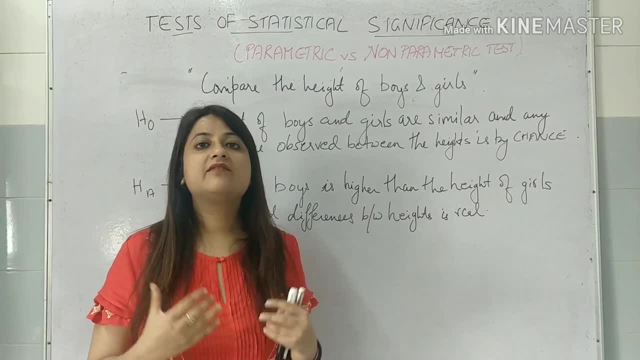 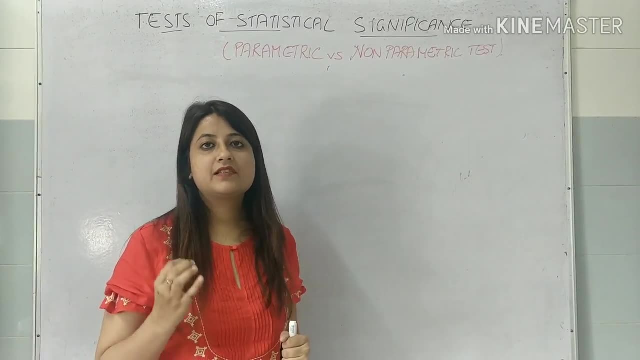 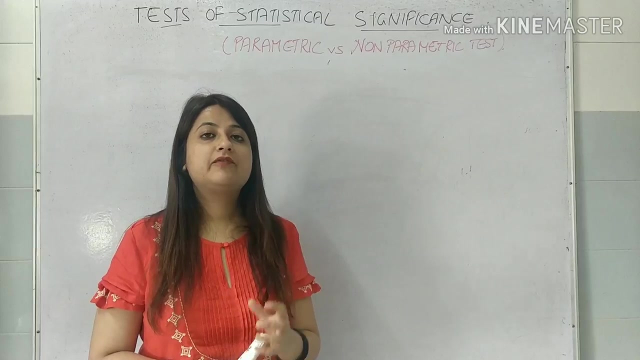 These are tests that help a researcher to confirm the hypothesis. So these tests of statistical significance, like I told you, helps the researcher to decide whether is hypothesis of true or not. Now there are lot of statistical tests, but for your MCQs, for your exams, what is needed is that these statistical tests will help a researcher to confirm the hypothesis. These statistical tests are divided into two main types. They are what I have written down: parametric and non-parametric test. So let us understand the difference between the two. So test of statistical significance is divided into two. 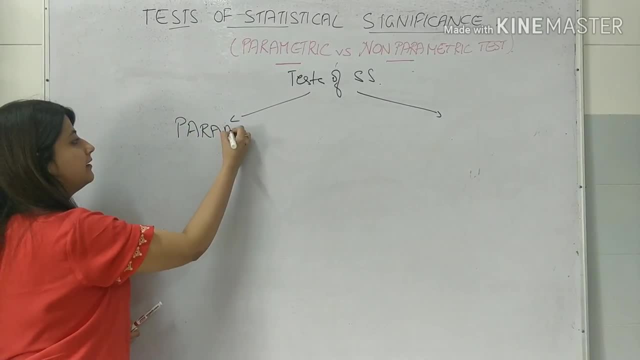 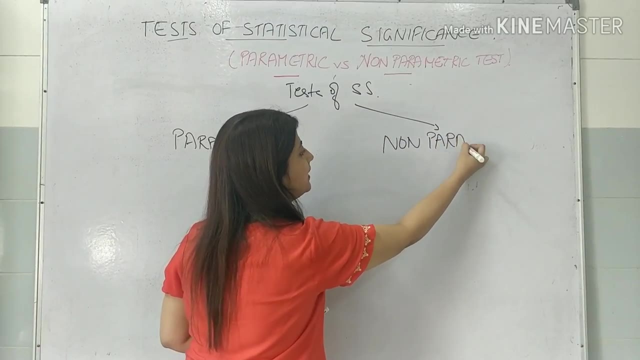 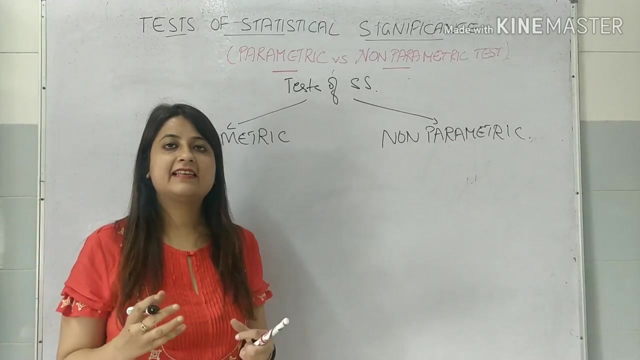 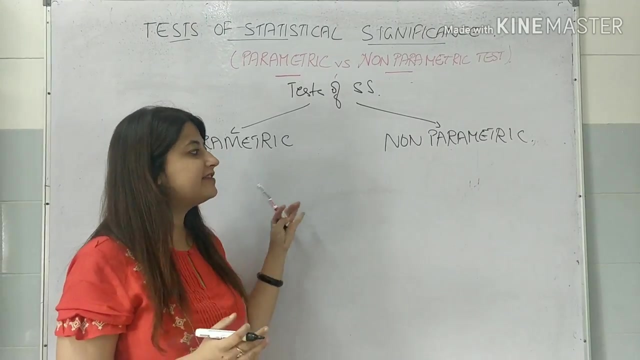 One is parametric test and the other is non-parametric test. Now, whenever you get an MCQ, you will get an example, you will get a situation and you will be asked that which test would you apply So for that? if you understand the difference between the two, it will be very easy for you to solve the question. So let us see what is the difference between them Now. parametric statistical tests are tests which are applied in a normal distribution, So the first difference is that parametric tests are applied when the distribution is normal. And, contrary to this, when will non-parametric test be applied? 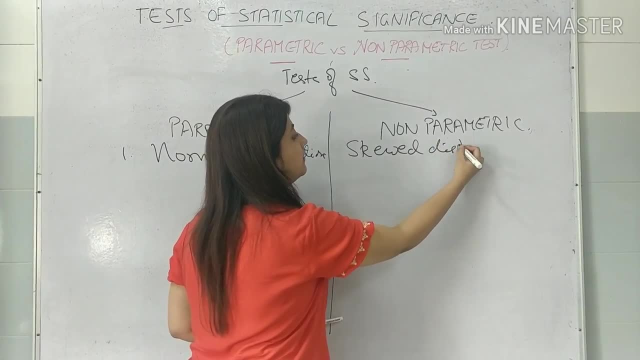 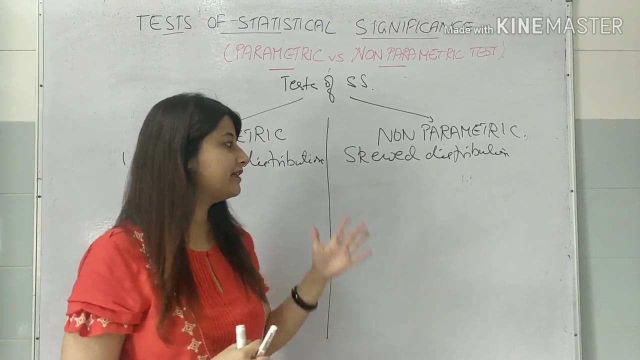 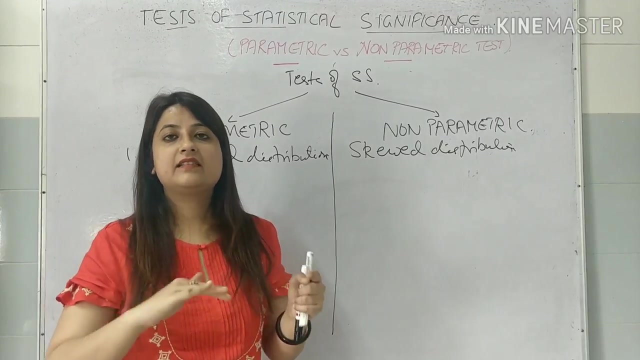 When we have a skewed distribution, Quick revision, normal distribution I have already discussed in my earlier videos. It means that mean is equal to median is equal to mode. All the three coincide. So skewed distribution is when my data is tilted to or my distribution is tilted to one side. So if the distribution is normal, we will apply a parametric test. If it is non-normal or skewed, we will apply a non-parametric test. So what is the other difference? The other difference? very easy, very simple: that parametric tests are applied for quantitative data. 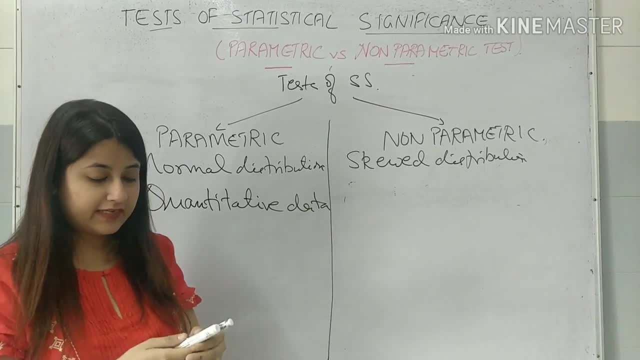 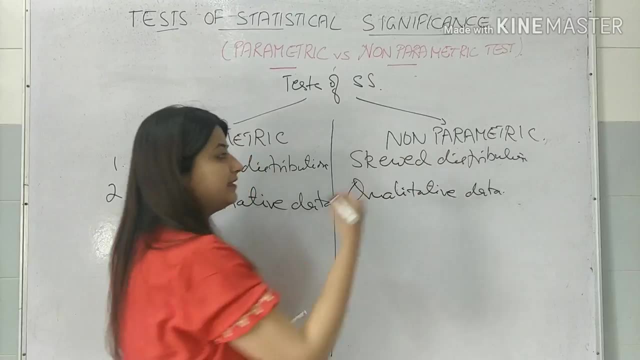 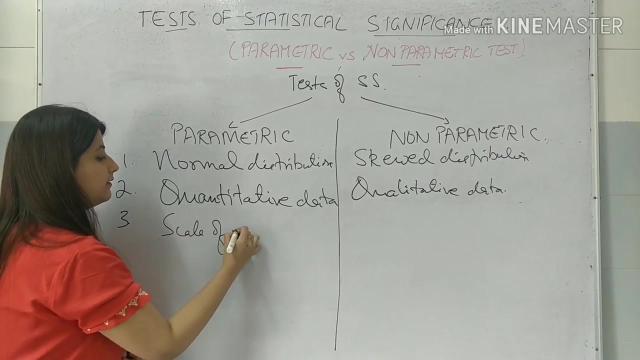 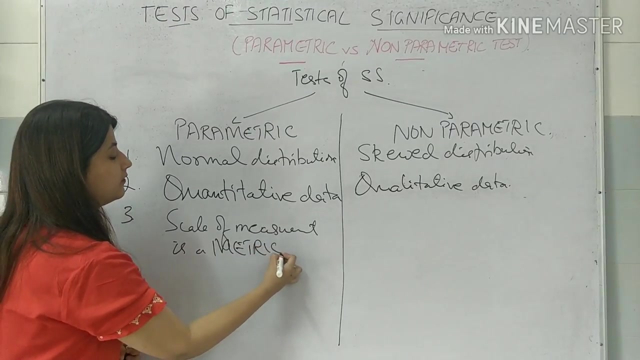 Non-parametric test will be applied when your data is qualitative. So this is my second difference. What is my third difference? A parametric test is applied when my scale of measurement is a metric scale. Okay, That means it is an interval. 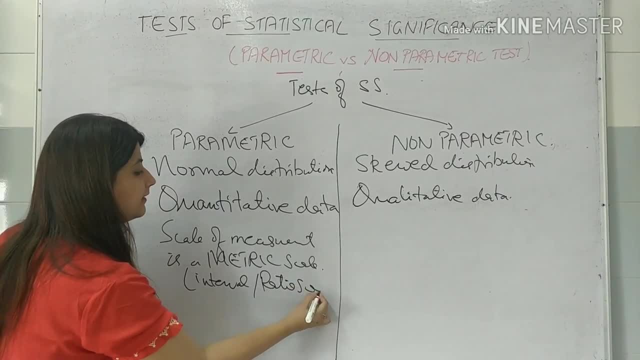 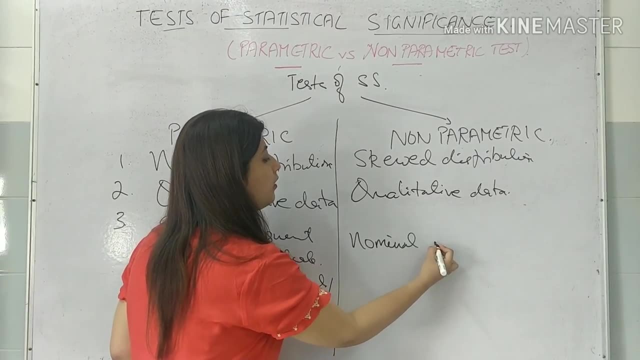 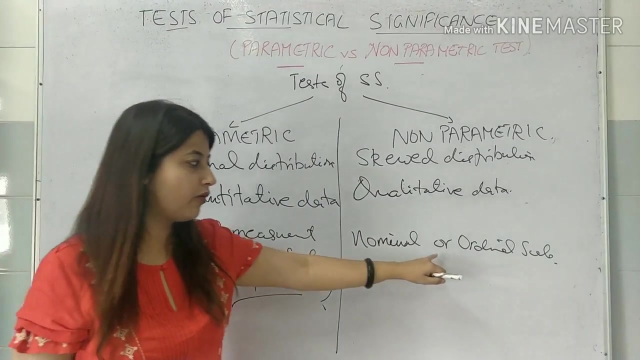 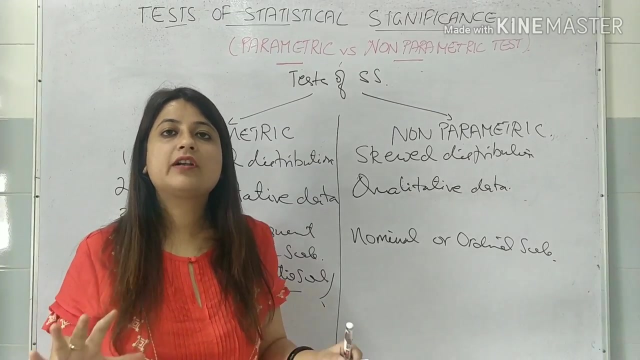 Or ratio scale. This we have already studied- And a non-parametric test is applied when we have a nominal or ordinal scale. Okay, That is when the data is being measured by using an ordinal scale or a nominal scale. Now, if you look at these three differences, you might still be thinking that I am not yet clear which test to apply. 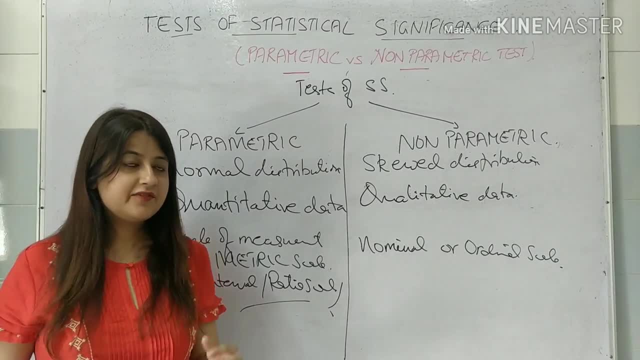 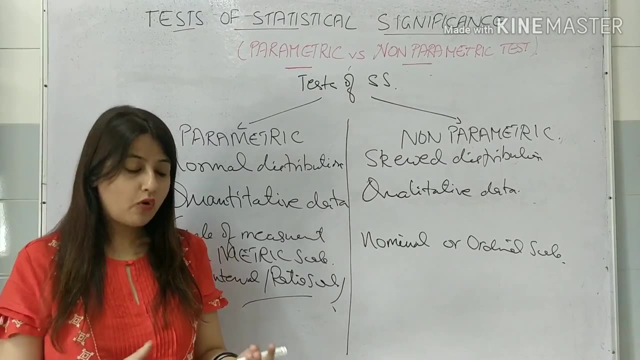 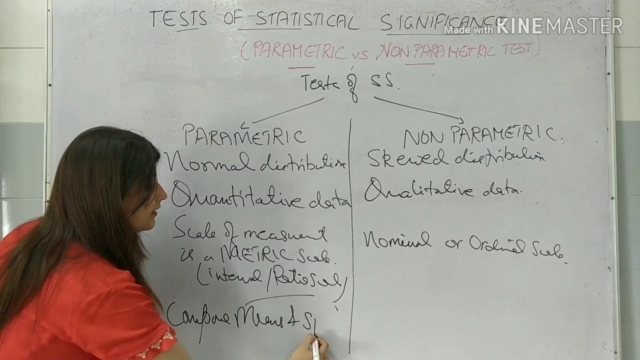 So there is a very simple way for this. So another difference is that if in your question you see that you are given means and STs or standard deviations, Or if you have to compare means and standard deviations, Then straight away we will apply a parametric test. 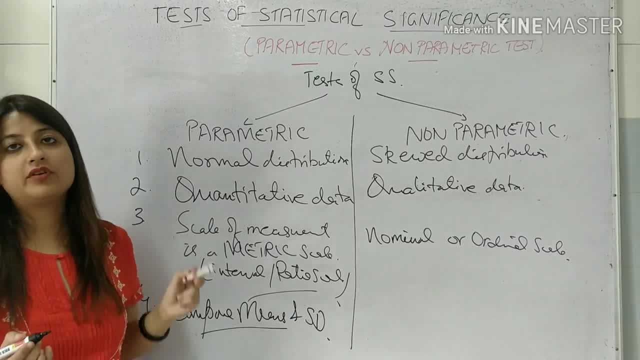 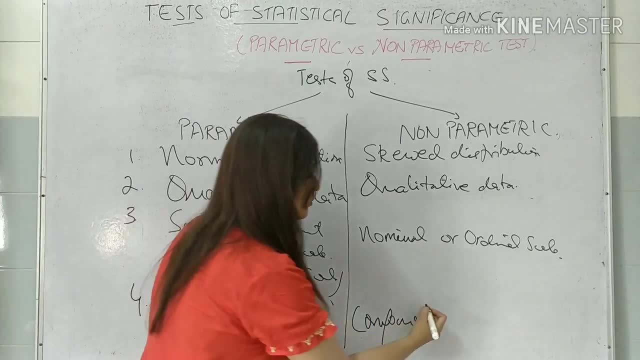 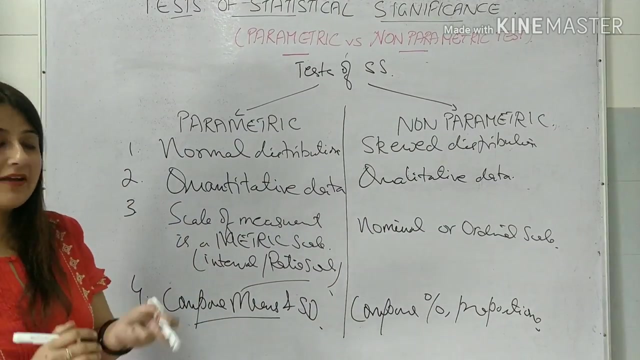 This is very important point to know in order to solve the interviews. And if, here, if you see that your question has percentages, proportions- Okay, Percentages and proportions- Then you have to use a non-parametric test. So you have to see in your question whether they are talking about means, STs, or percentages and proportions. 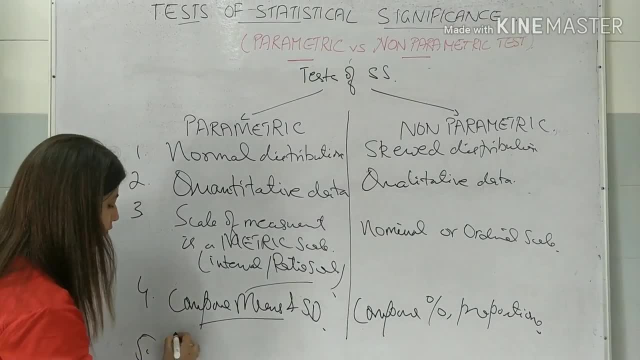 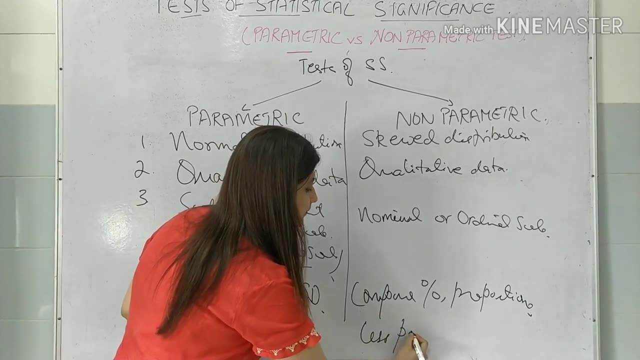 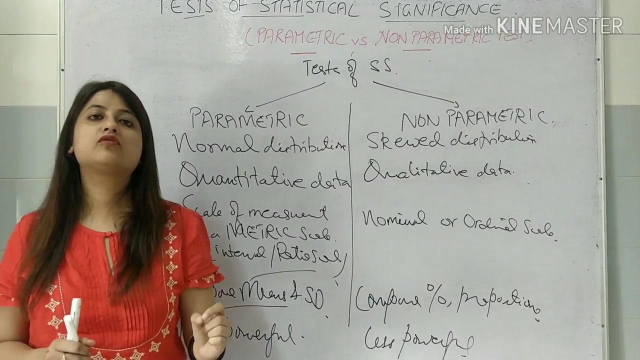 The last point is that parametric tests are more powerful than non-parametric tests, So this can also come as a university question. These are the main differences. To be able to solve your MCQ, please remember, if you are given means and STs, you will use parametric tests. 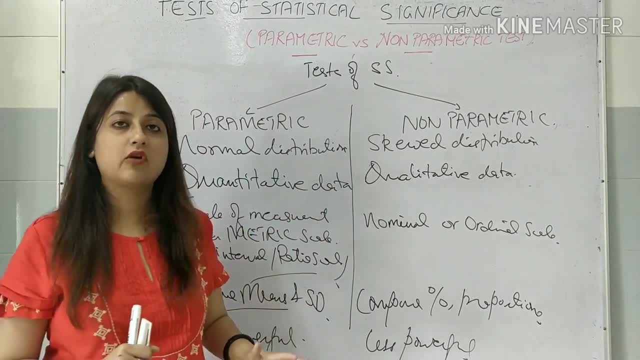 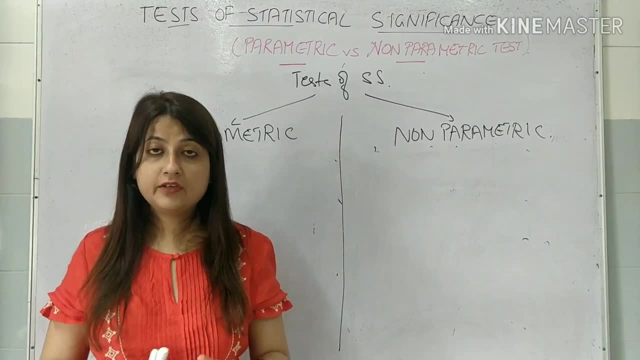 If you are given percentages and proportions, you will use a non-parametric test. Now let us see some of the important parametric and non-parametric tests that you need to know to solve MCQs. Some of the parametric tests that you should know are: 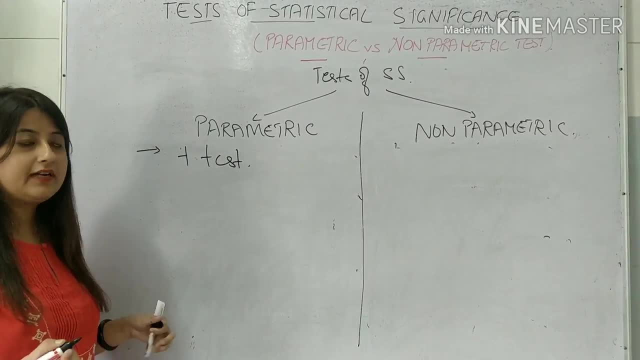 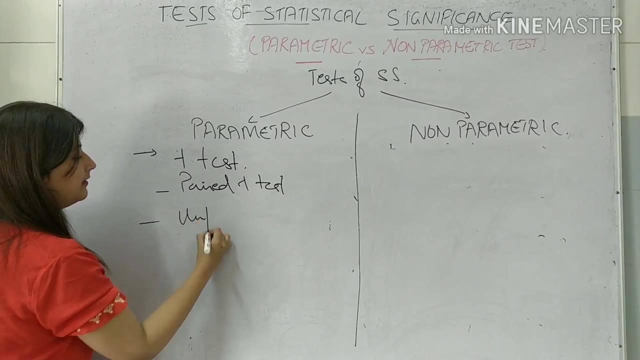 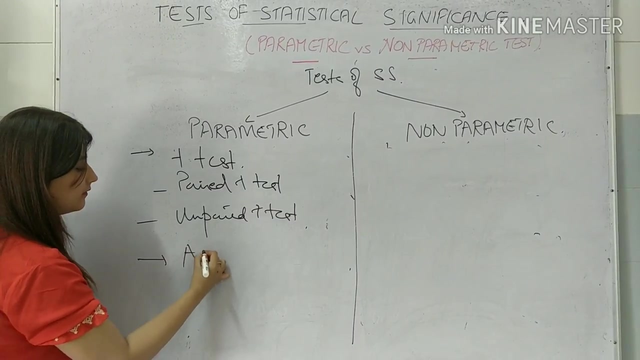 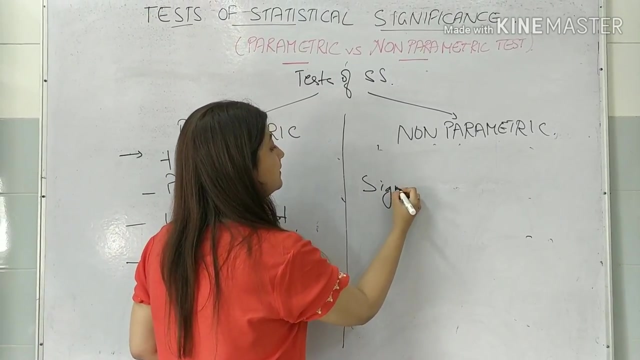 T-Test, Student T-Test it is also called. In this you have paired T-Test and Unpaired T-Test And the other parametric test that you should know is Unovercome. The non-parametric test that you should know is: 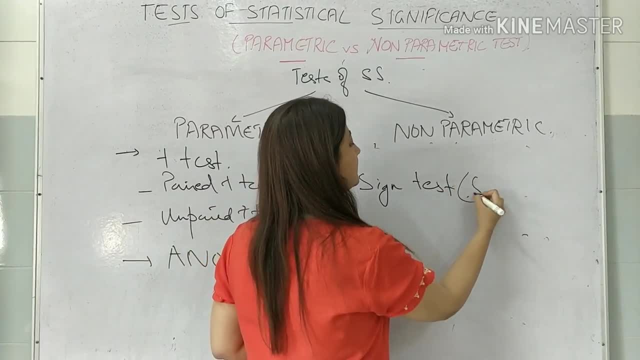 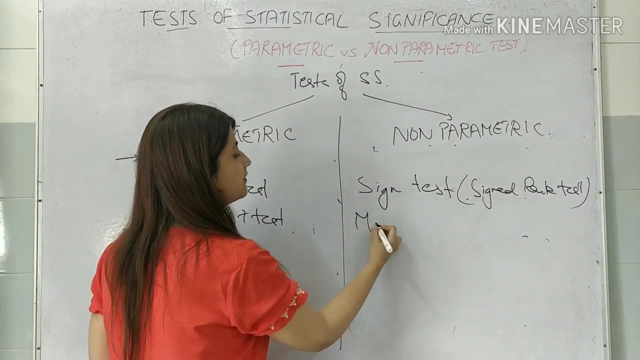 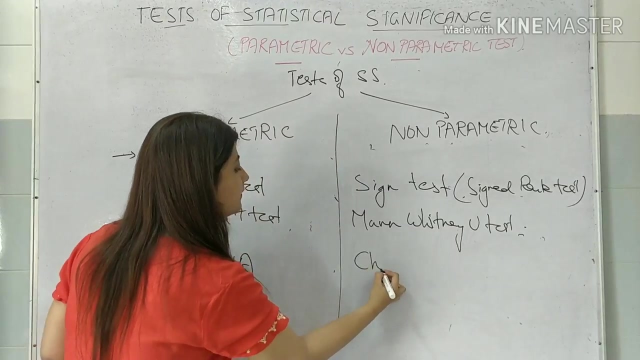 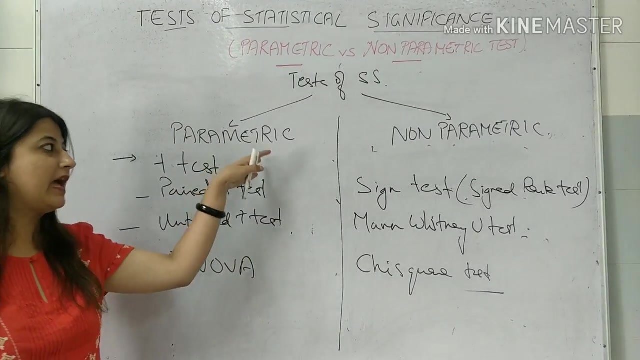 Sign Test or you also have Sign Rank Test. You also have Mann-Whitney U-Test And you have Keiswell Test. Now they can give you an MCQ. that ANOVA is a parametric test, non-parametric test, some of the other options. 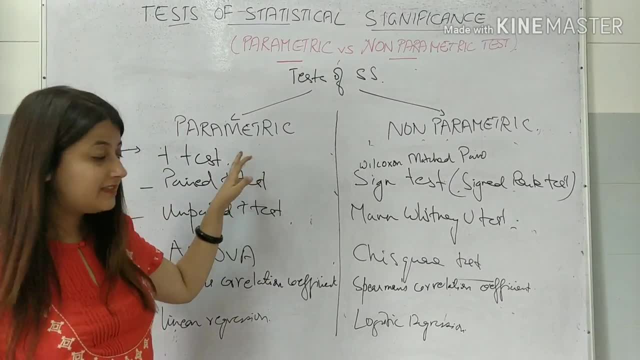 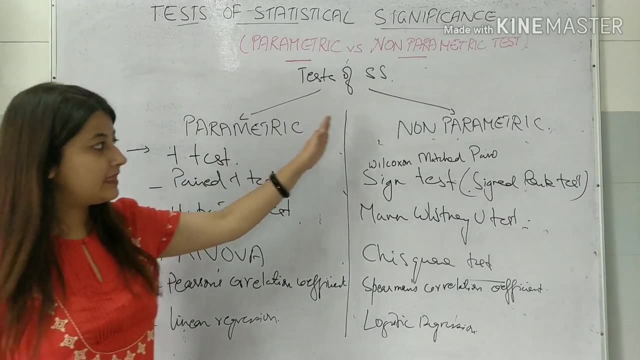 So this you need to know. So these are my parametric tests: T-Test where you have paired unpaired ANOVA, Pearson's correlation coefficient, linear regression. These are my non-parametric tests. You have Wilcoxon Mashed Pair Sign Rank Test. 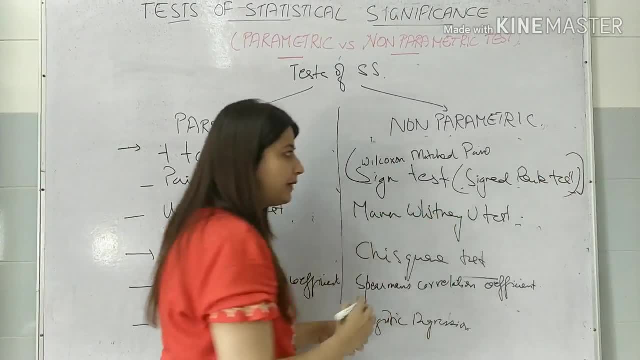 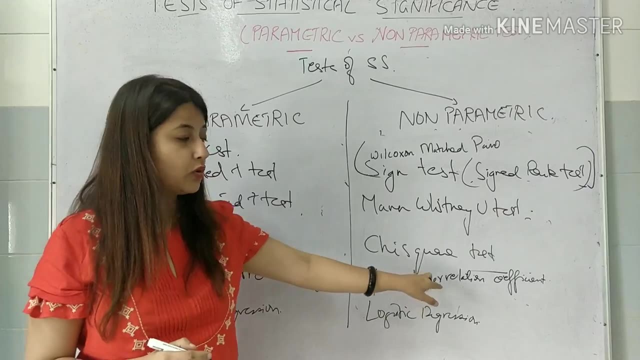 Once they had written this full name in an aims paper and students got confused. We have Mann-Whitney U-Test, We have Chi-Square Test, We have Spearman's correlation coefficient and logistic regression. Now all of these are counterparts of each other. 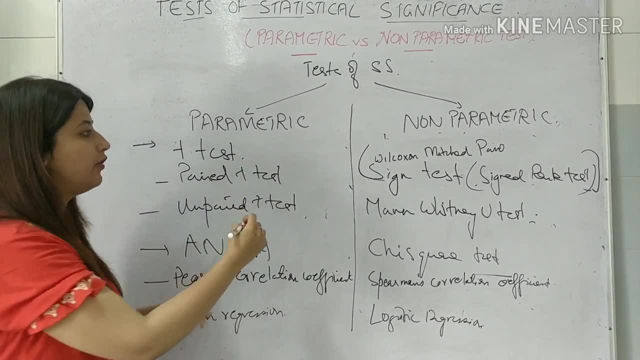 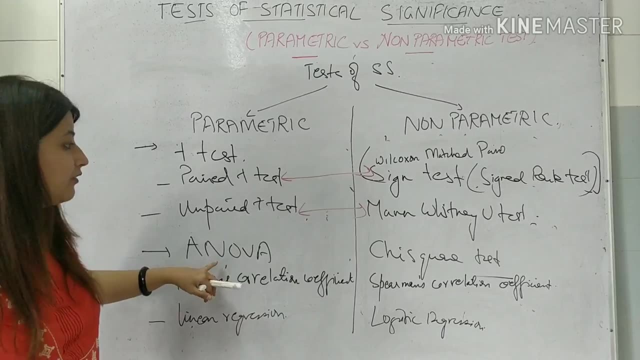 Like for parametric, the counterpart of paired T-Test is sign test. Okay, For unpaired T-Test it is Mann-Whitney U-Test. For ANOVA, we can have Chi-Square And also Chi-Square. one other test. 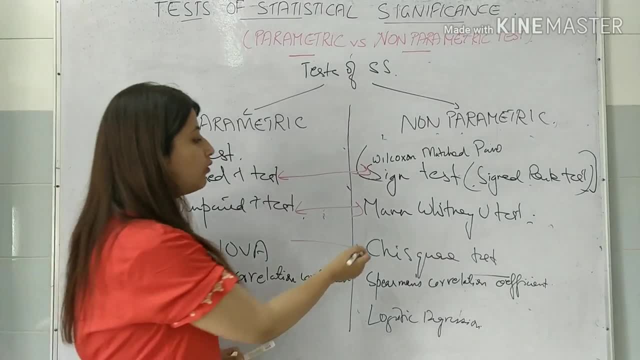 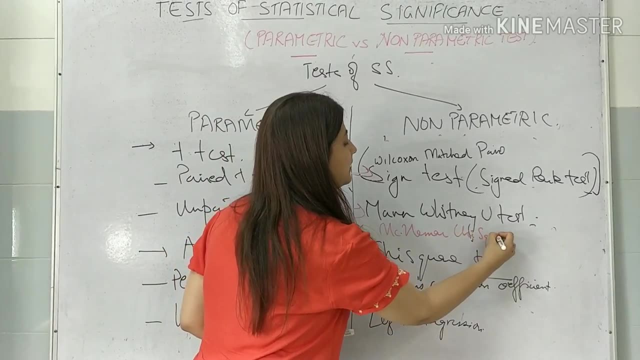 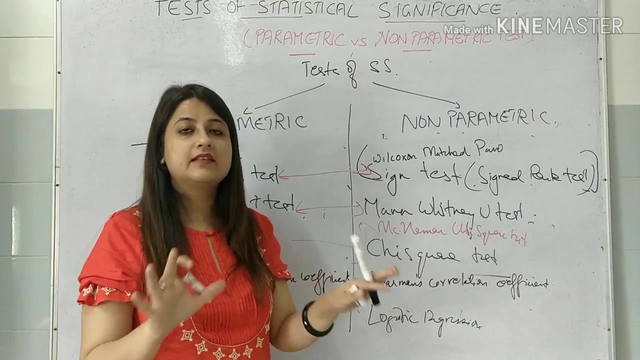 McNemar Chi-Square Test, Which is also a counterpart of unpaired T-Test. That is McNemar Chi-Square Test. But this is too much logical, Too much hi-fi. I would say This is: even if you forget, it will do. 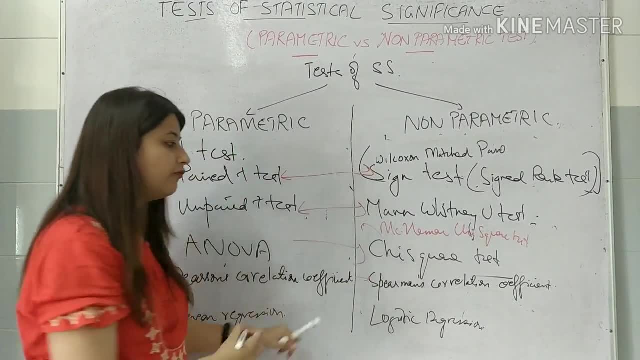 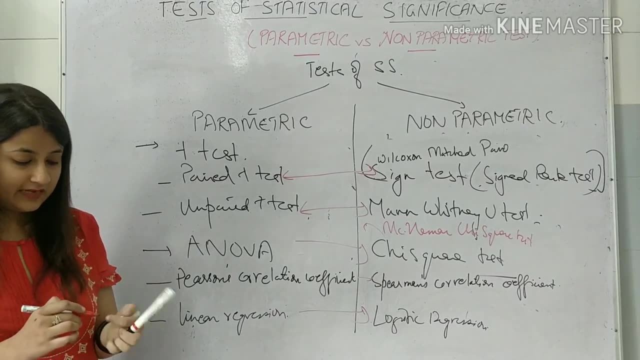 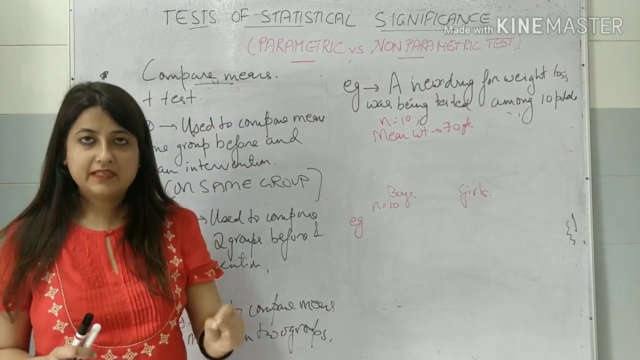 Pearson correlation coefficient- you have a counterpart. Spearman correlation coefficient. Linear regression: you have Linear regression. you have logistic regression. So you must at least know the names. Now let us try to understand. what is T-Test? Okay, Whenever you have to compare means. 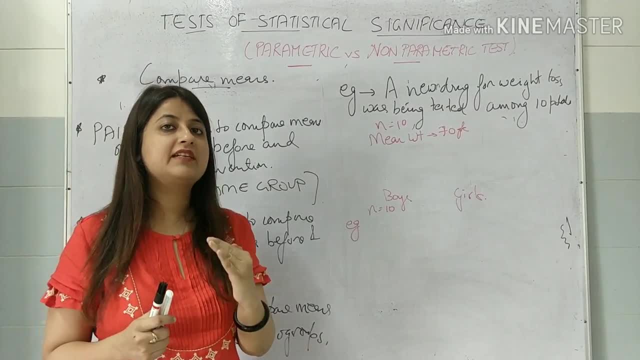 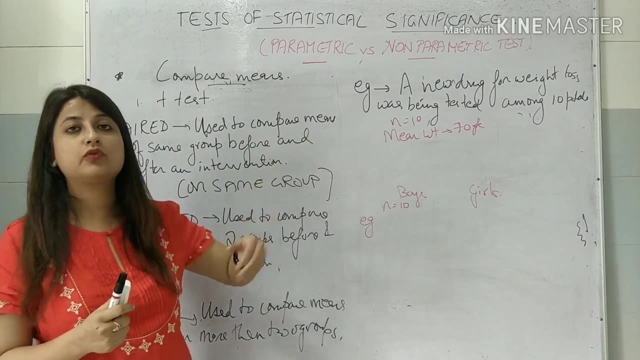 Then you will be using a T-Test, A student's T-Test. Now it can be paired or it can be unpaired. What do you mean by paired? Paired means that it is used to compare. Paired is actually before and after. 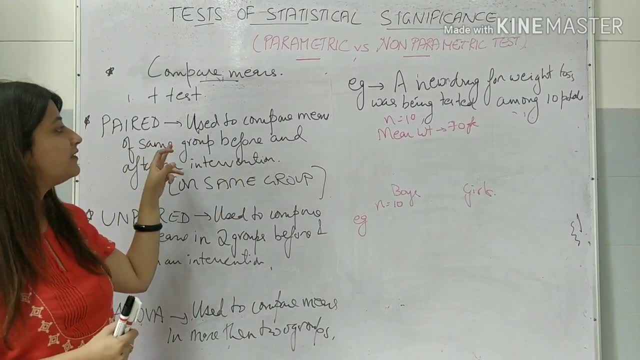 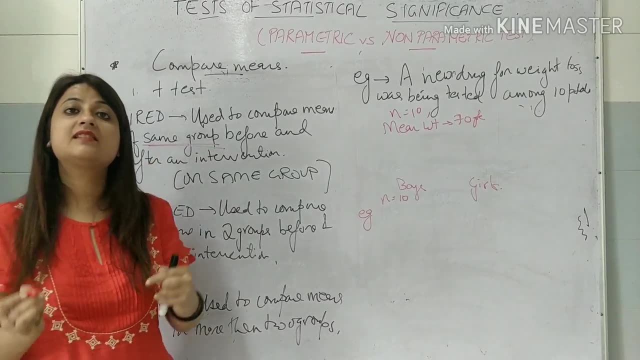 Okay, But here it is. It is used to compare means of the same group before and after an intervention. So for paired T-Test, the thing is that you are doing it on the same group. Unpaired T-Test is: this is also used to compare means, but in two groups. 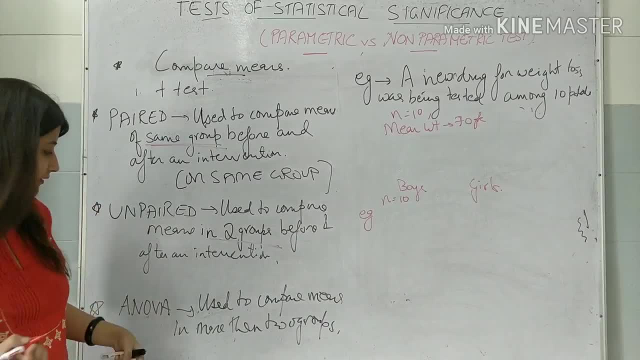 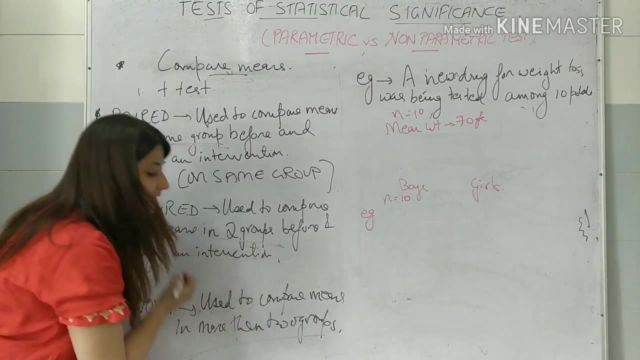 You are doing it in two groups before and after an intervention, And Anomaly is analysis of variance In this. you are used to compare means in more than two groups. Let us try to understand with an example. First let us look at a paired T-Test. 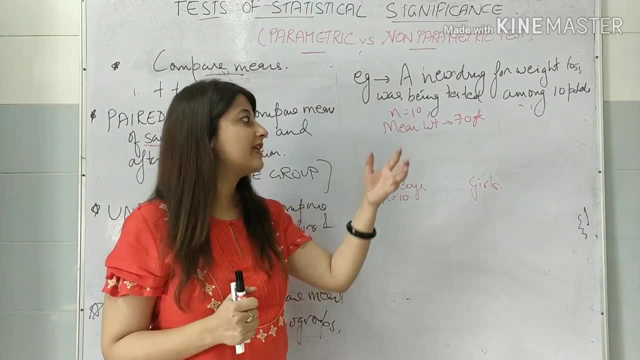 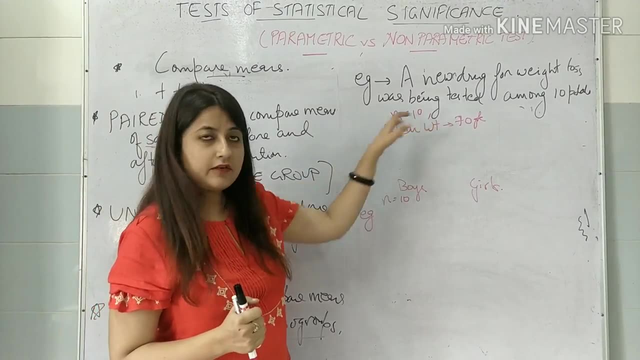 Suppose you have a question or you have an example, like A new drug for weight loss is being tested among 10 patients, Okay, So n equal to 10.. The mean weight of that group is, say 70 or say 100 kgs. 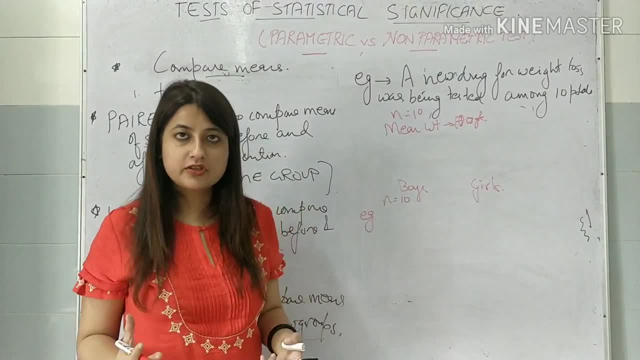 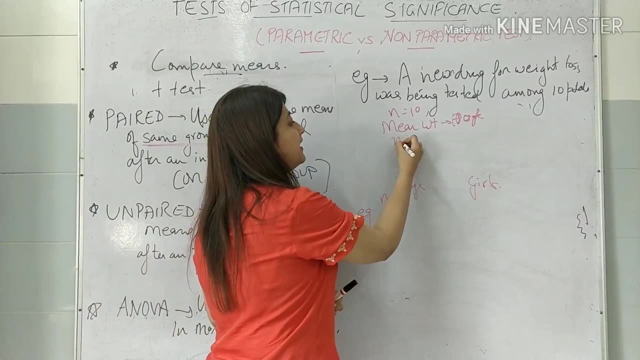 Okay, Suppose this is 100 kgs. Now I have launched a drug And I want to see what is the effect of that drug on the weight of these 10 people. So I will give that drug, say, for 3 months. Okay. 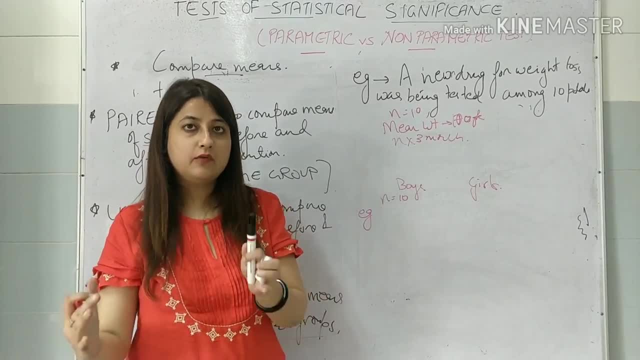 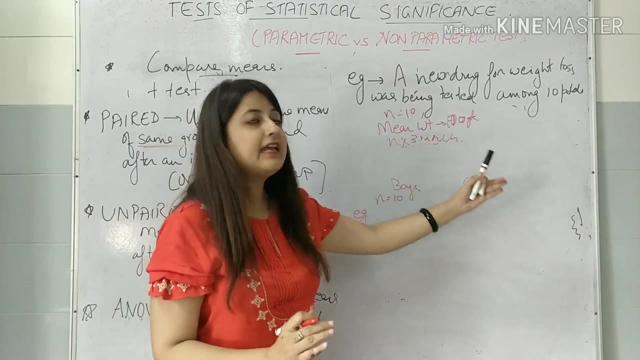 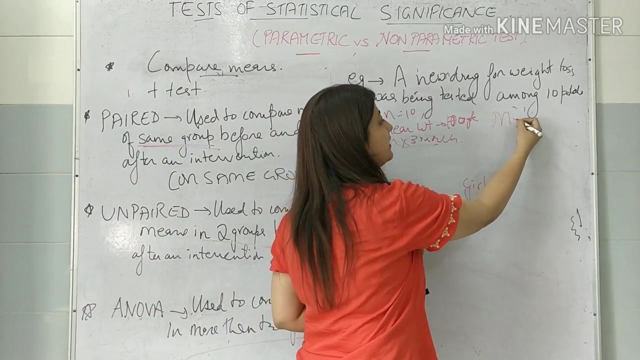 Again, I will take their weight. So what am I doing? I am recording their weight before giving this drug, Before the intervention. Again, I will record the weight, Mean weight After giving this drug for, say, 3 months. Then my mean weight comes out to be, suppose, 60 kgs. 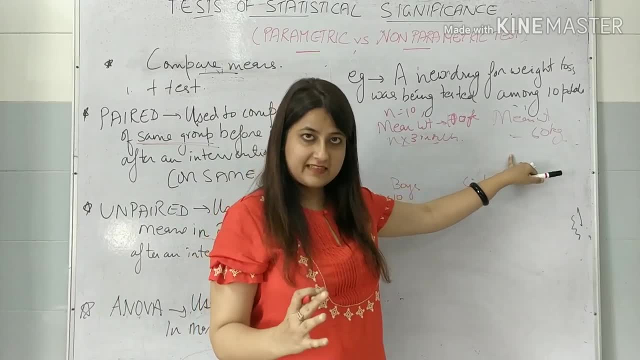 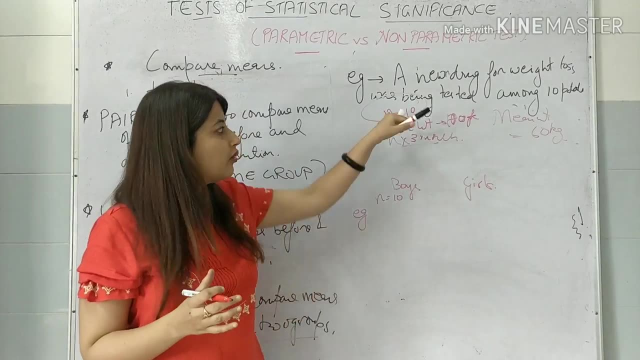 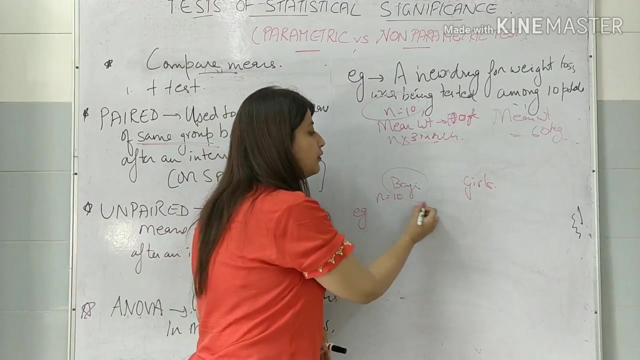 Okay, But whom am I testing this drug on? On these same 10 people. So I am doing this drug, This testing of the drug, on the same group of people. So this becomes a paired t test. Now for an unpaired t test. suppose I do it in 2 different groups. 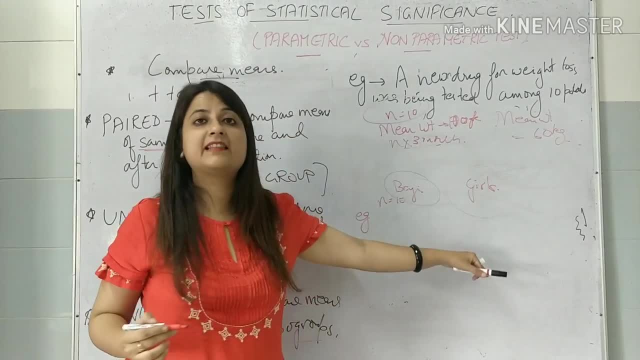 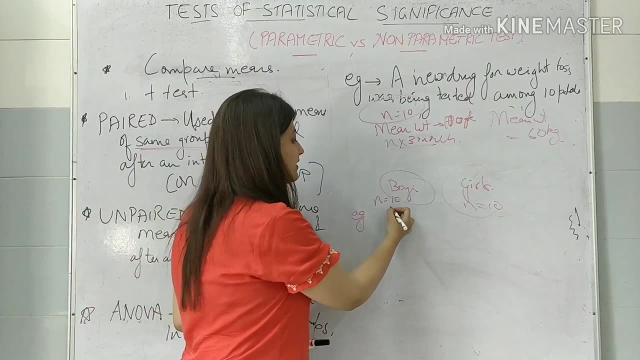 Boys and girls. I do not compare their weights. Here I have 10 boys, Here also I have 10 girls. Okay, Here the mean weight of the boys is, say, 160 kgs. I give the drug for, say, 3 months. 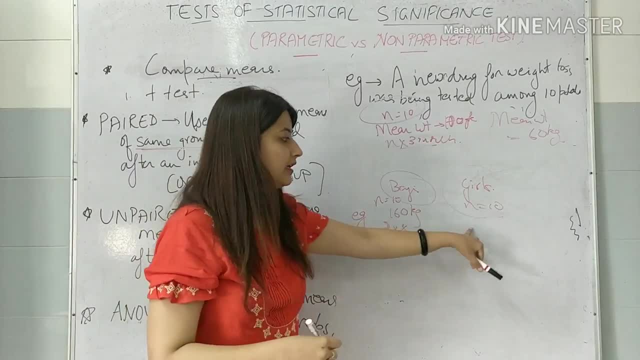 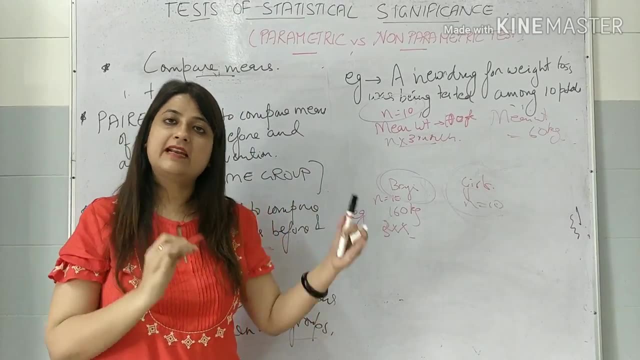 Okay, Then again I record their weight. Similarly, I do it for girls. So what am I doing? I am comparing the means of 2 groups before and after an intervention, So this becomes an unpaired t test. Now suppose I have more than 2 groups. 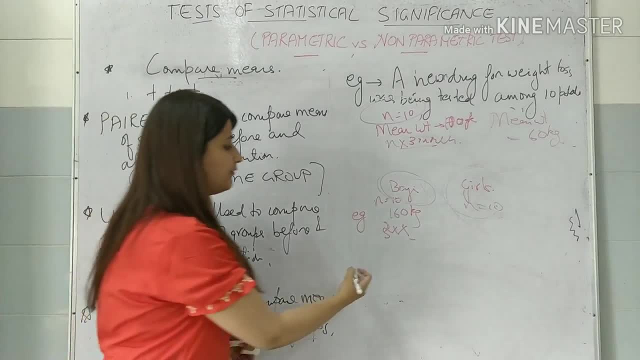 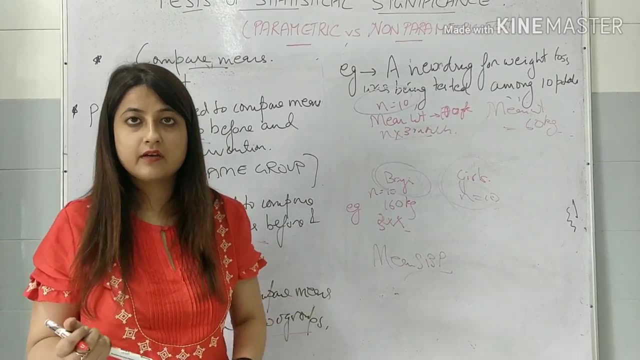 Suppose I have 3 groups, 30 groups. Suppose I have to consider the mean systolic BP of patients in, say, surgery ward. Okay, I have different number of wards, So in that case it will become which test we will use? ANOVA test. 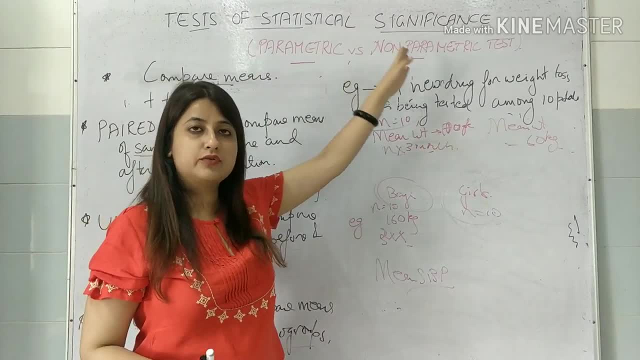 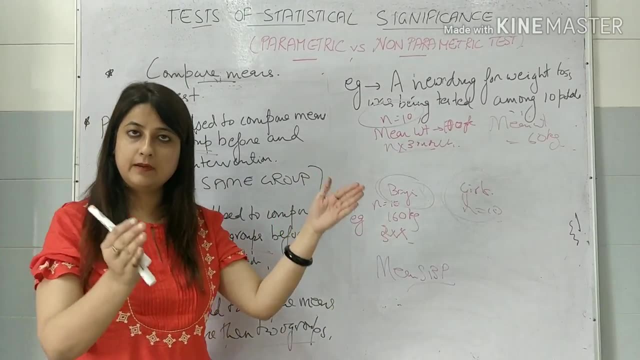 So if you are questioning now, you need to first figure out whether you need to use a parametric test or a non-parametric test. Since the question involves mean weight, it is clear that you will be doing a parametric test Now out of that, which test out of these 3?? 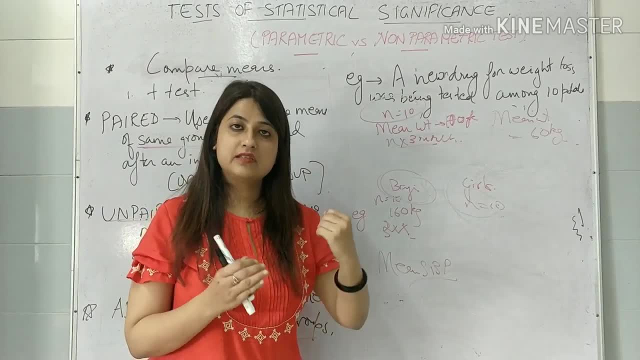 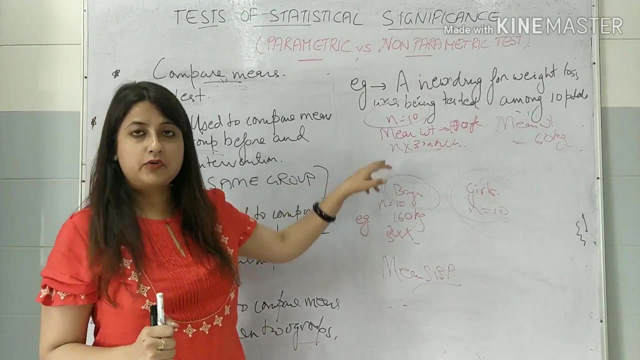 So you have to see whether you are doing it on the same group, you are doing it on 2 different groups or you are doing it on more than 2 groups. Now, the counterpart I told you of paired t test was Simon test. 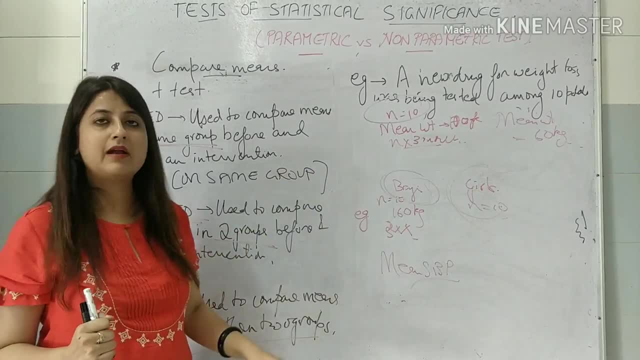 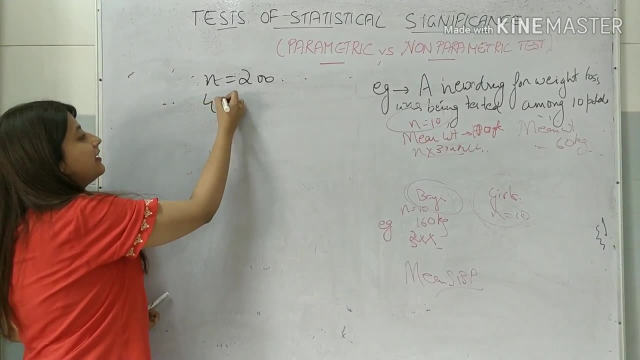 Right And of unpaired t test was Mann written u test. So just to understand, I will give you one example. Now suppose we have a group of 200 people, Okay, And out of that, say, 40% are diabetic. 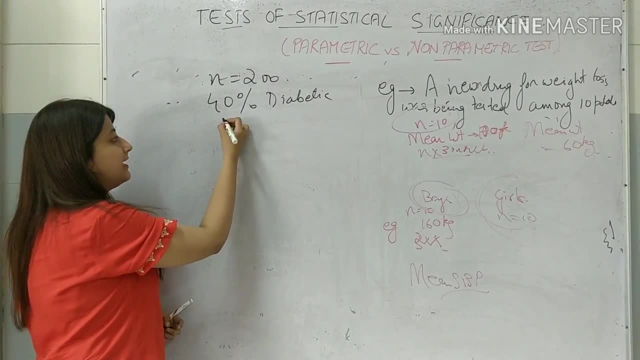 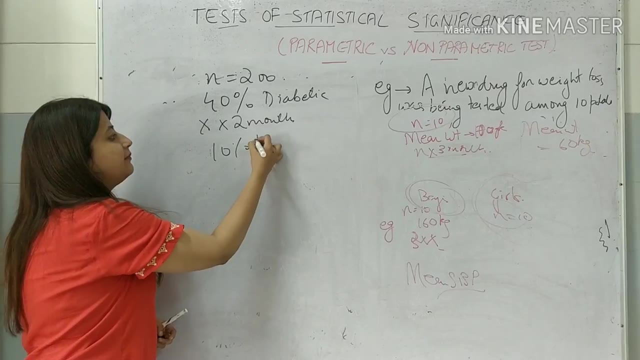 Okay, Now I give a drug and that drug I give it for 2 months. X is given for 2 months. Now I see that after taking that drug for 2 months, only 10% are diabetic And I ask you: 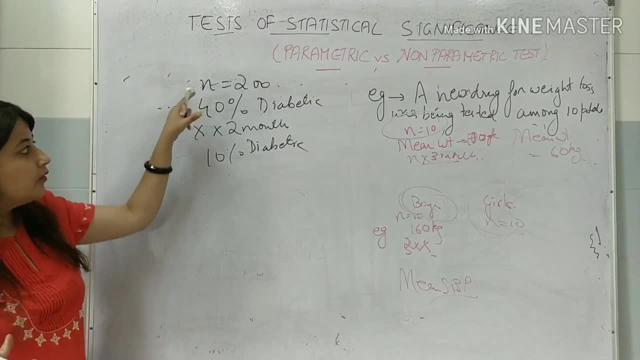 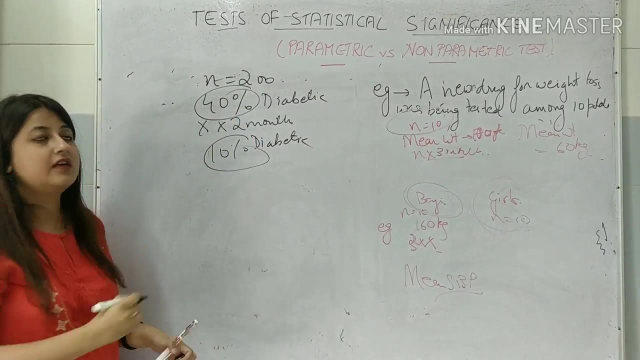 Which statistical test of significance is used. Now what will you see? First I told you that look at the values. Here the thing is giving in percentages, So you are clear that this is not for parametric test. We cannot apply. 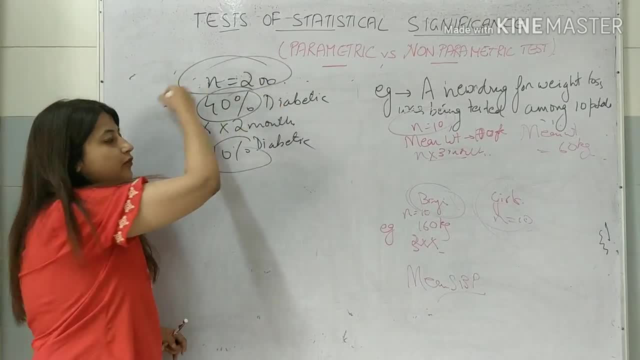 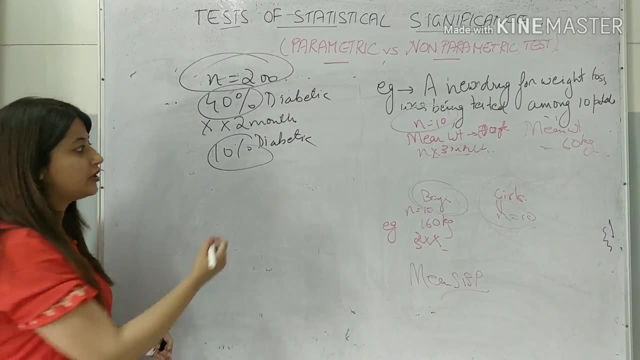 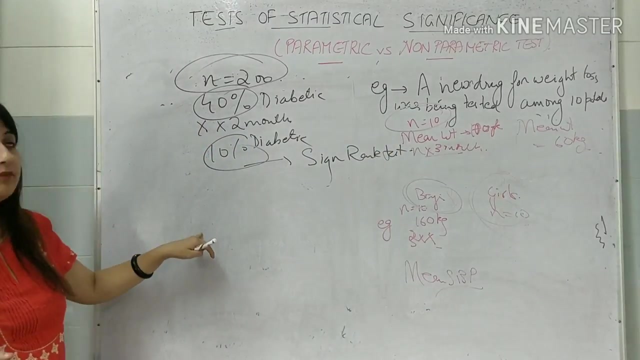 This is a non-parametric test And we are doing it in the same group of people. So this is a non-parametric test, A counterpart of paired test, Which I have told you is a sign ran test. Okay, Now suppose the same question was: I have n equal to 200.. 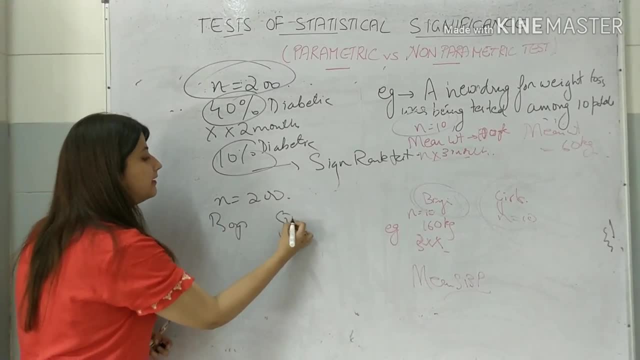 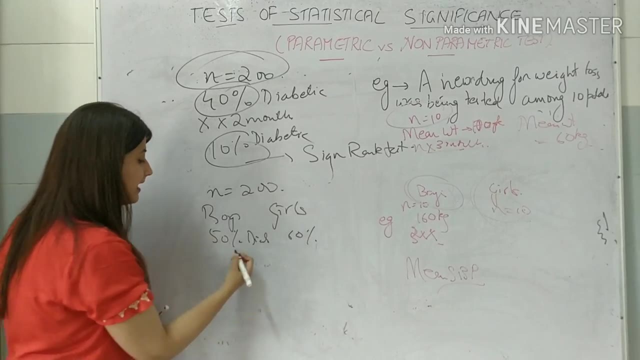 I have two groups, Boys and girls, Or males and females, And in this there are 50% diabetic, Here there are 60% diabetic. I take the drug for 2 months Now. here 10% remain. Here, say, 5% remain. 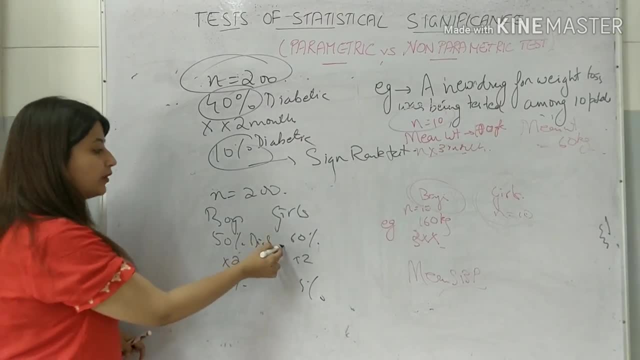 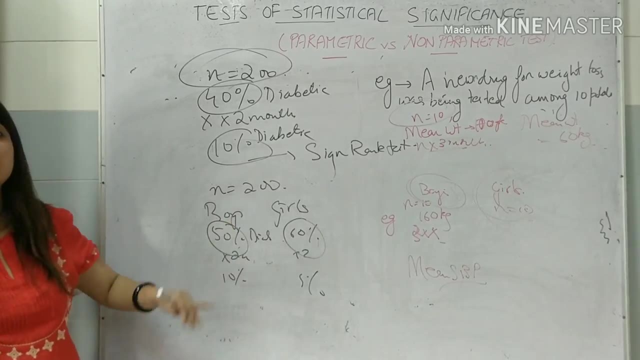 So which test will I use Now here? what am I doing? I am doing it. I am comparing percentages and proportions, So it automatically becomes a non-parametric test, And I am doing it for two groups, So it will be a counterpart of unpaired t-test. 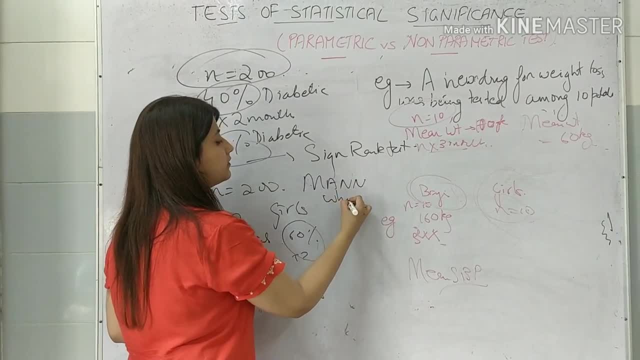 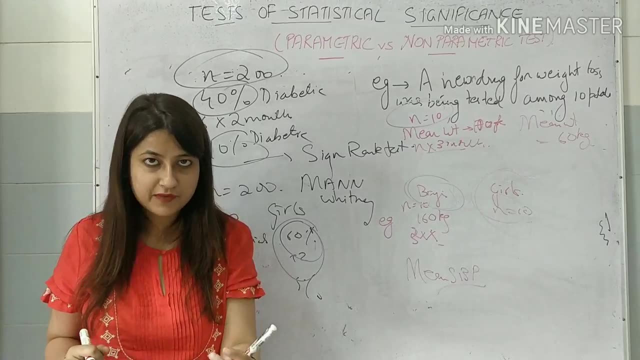 Which I told you was a man-minty-you test. Also, since you are dealing with proportions and percentages, You can also use chi-square test In the form of test of association, Which we will discuss in our next video, When I will in detail teach you.